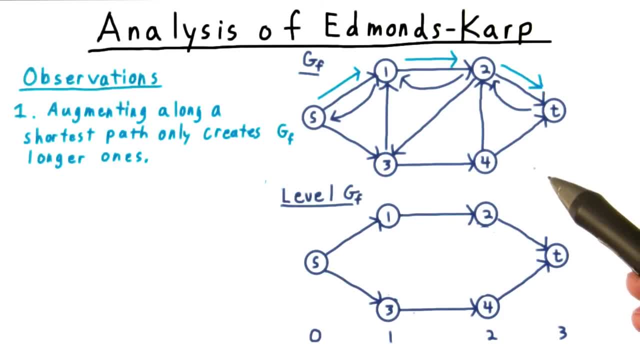 Note, however, that these edges are useless for creating a path of the same length. In fact, because they go back up a level, any path that uses one of them must use two more edges than the augmenting path that we just used. 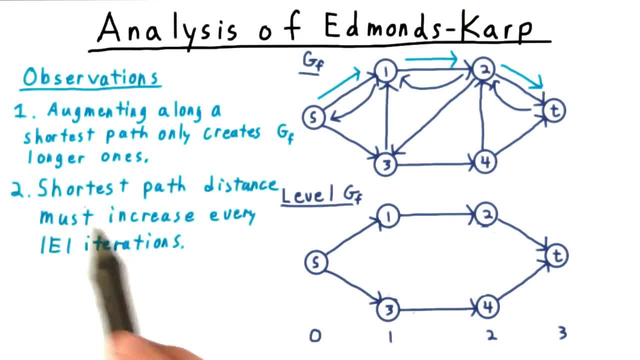 the one that was the shortest path. Next, we observe that the shortest path distance must increase every e iterations. Every time that we use an augmenting path, we delete an edge from the level graph, the edge that got saturated. This one here got saturated in an augmentation along this path. 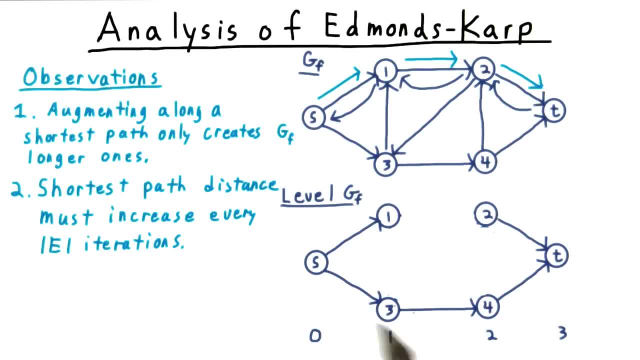 so we would delete that. Then maybe we push another flow along this path and end up deleting this edge. These edges won't come back into the level graph until the minimum path length is increased. As we've already argued, the reverse edges are useless until we are allowed to use longer paths. 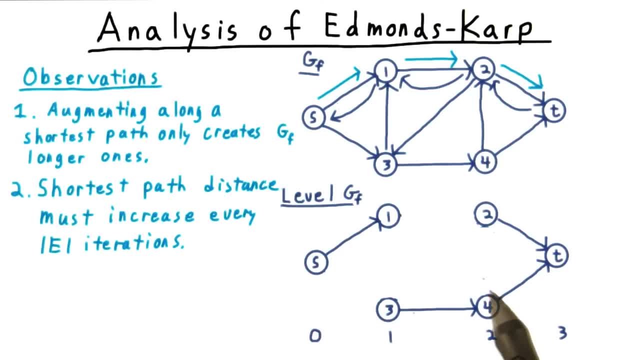 If each augmentation deletes one edge from the level graph, then certainly after e iterations, the level graph would be empty. Obviously, there are no ST paths in this level graph, and so we need to build a bigger one that includes longer paths in order to be able to augment any further. 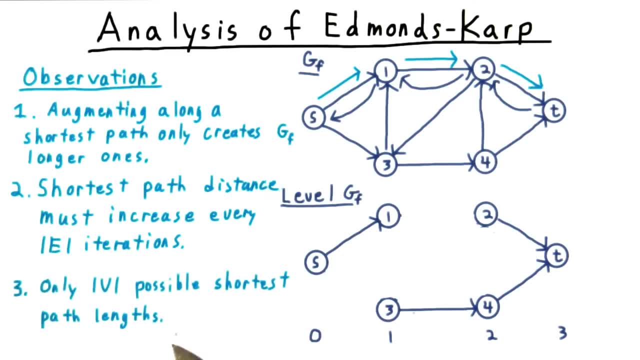 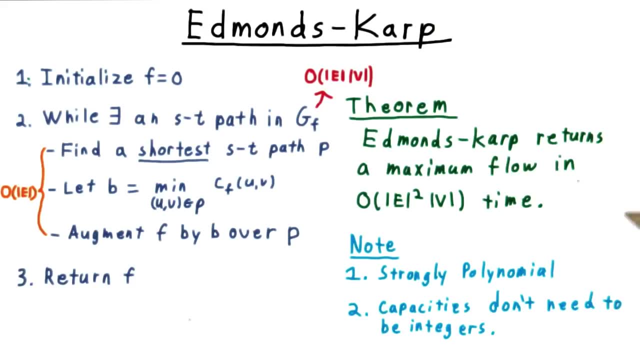 Lastly, there are only V possible shortest path lengths, so that completes the theorem. For each possible path length we might have up to e iterations. Going back to the theorem, note that we've eliminated the dependence of the running time on the capacities.